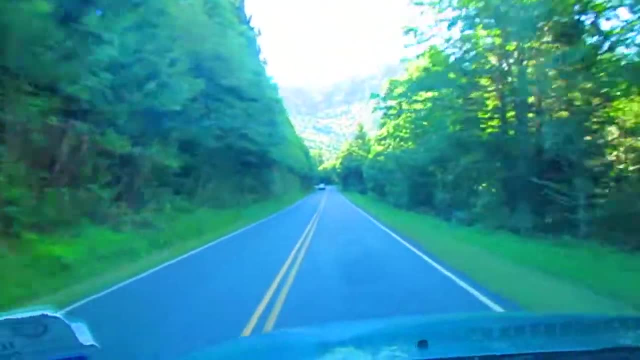 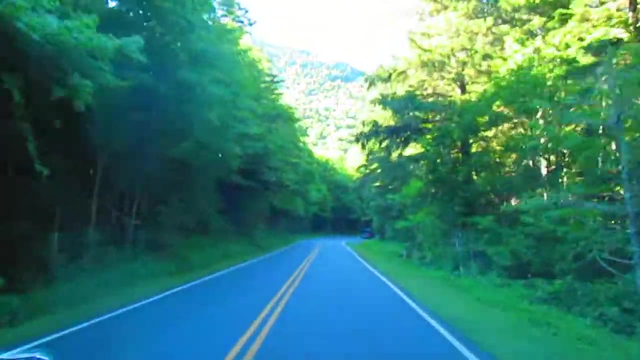 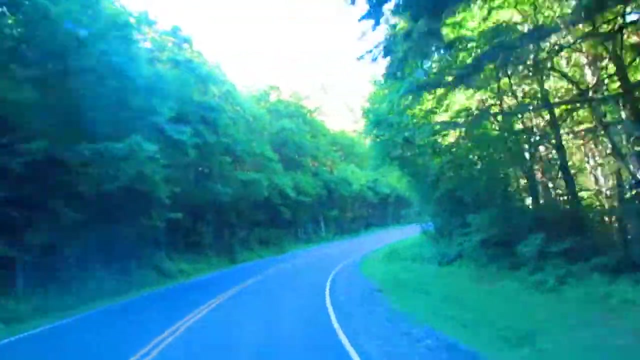 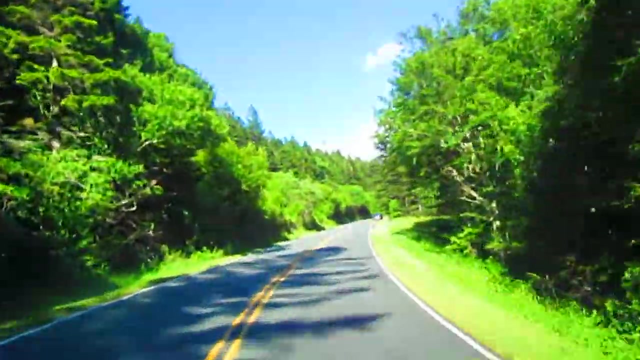 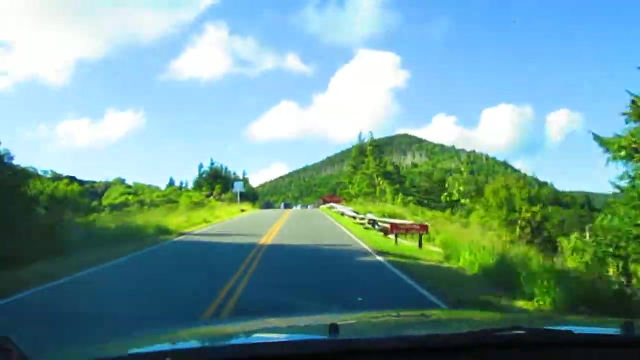 Really great views, beautiful highway. That's about 3 miles from the Blue Ridge Parkway to the camping area and about 5 miles to the top of the mountain where there's a little restaurant and observation tower. Okay, here's the entranceway. 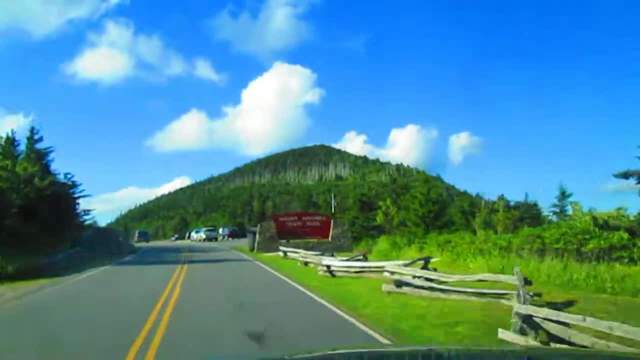 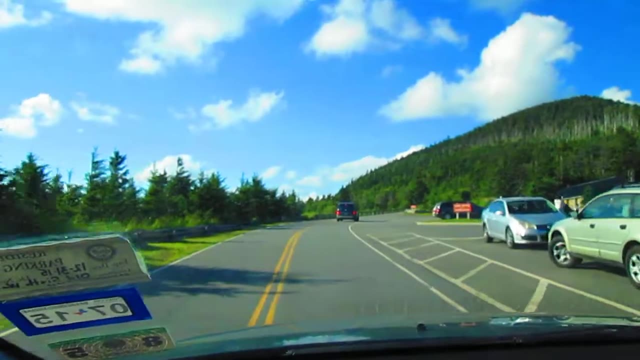 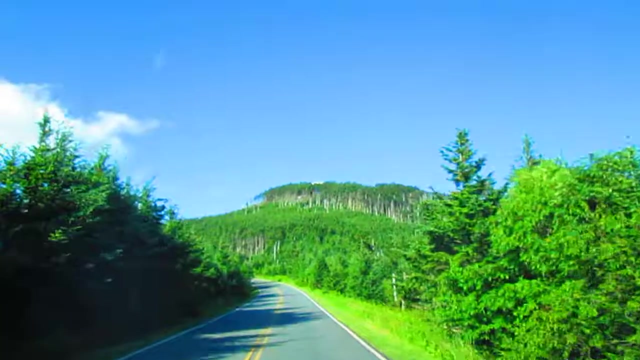 It takes a long time to drive this Blue Ridge Parkway because you're always stopping and taking pictures of things. This is really pretty here. This is awesome. Let's go find out what's the story here. You can see the tower up there. 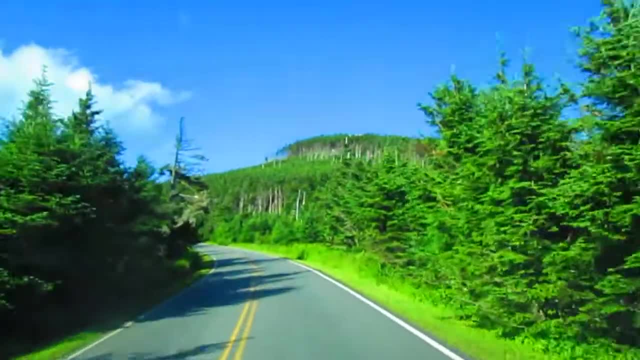 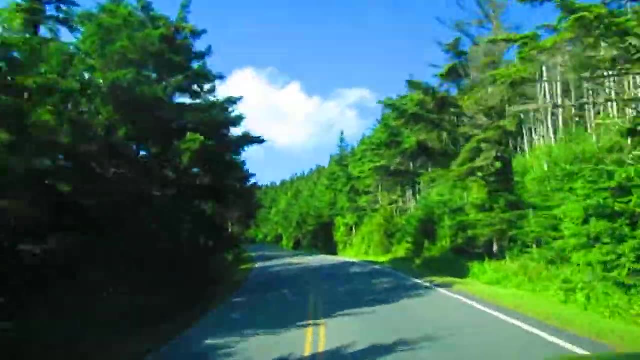 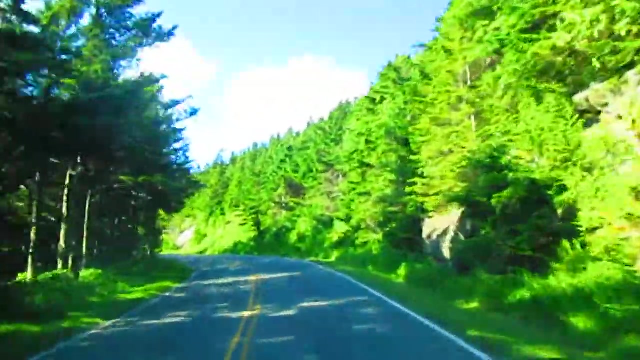 It's really beautiful out here. It's very high up with outstanding views. It's very high up with outstanding views. It's very high up with outstanding views. It happens to be a really clear day today. It's a beautiful drive on the Blue Ridge Parkway and then up to the mountain here. 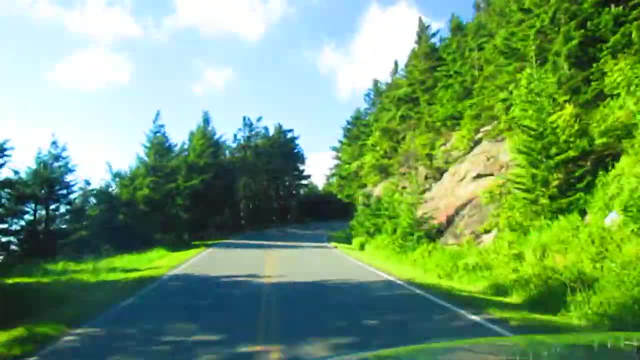 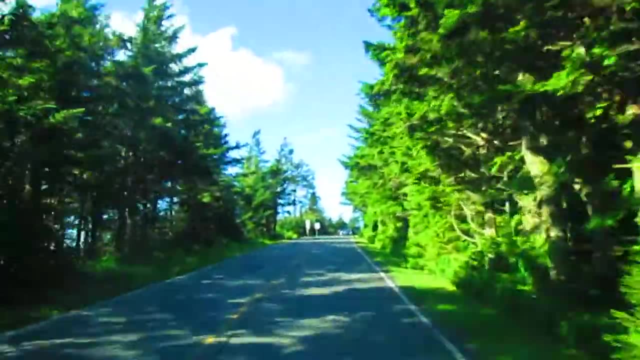 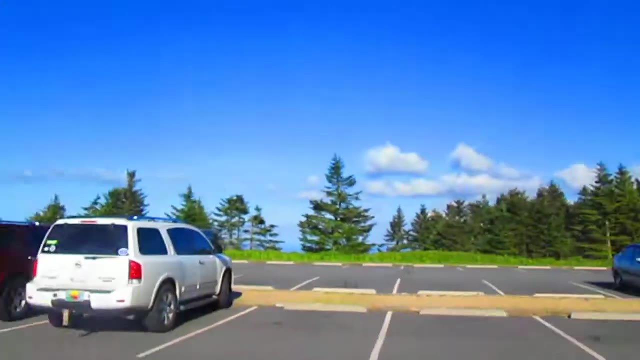 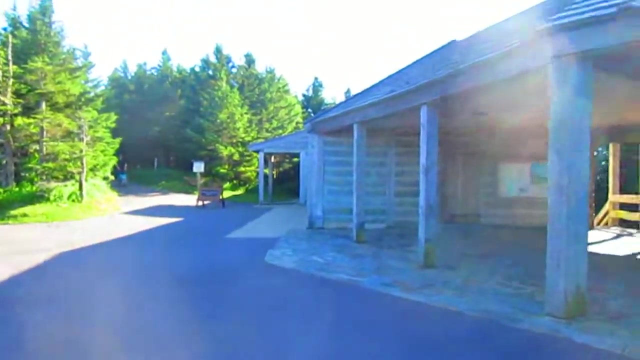 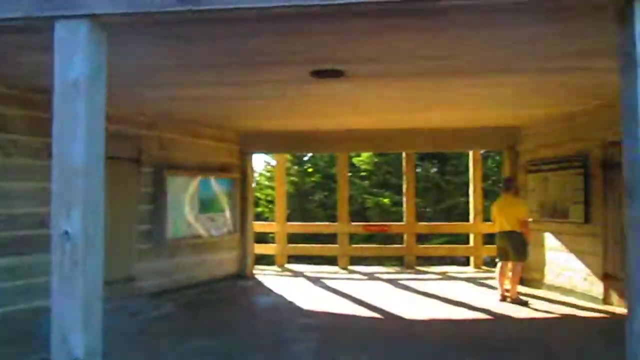 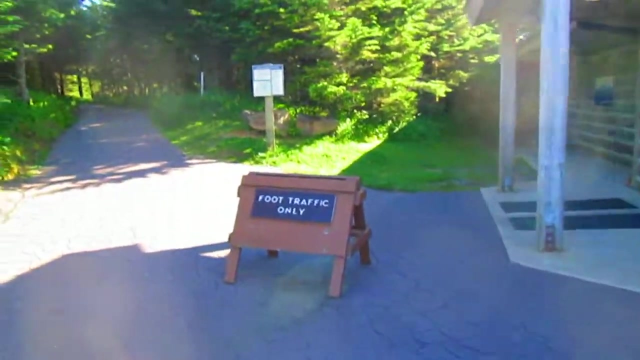 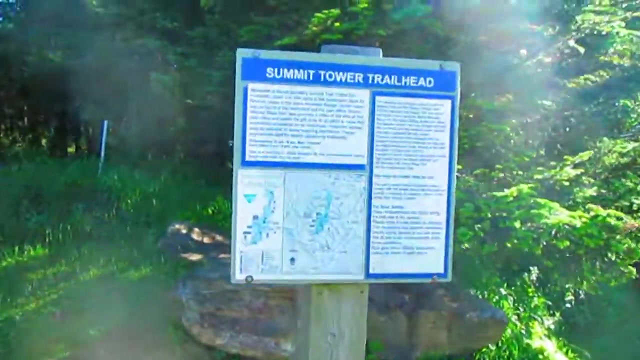 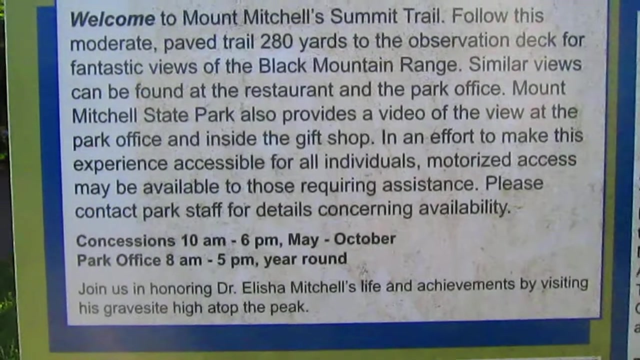 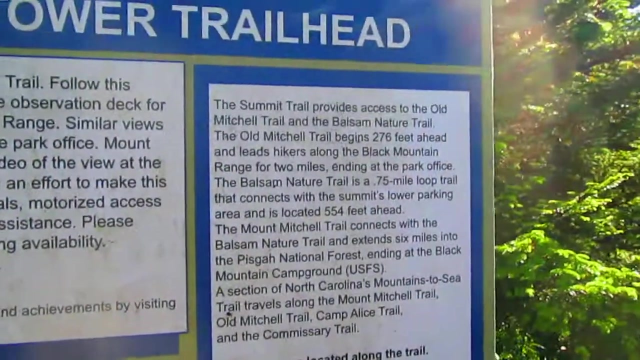 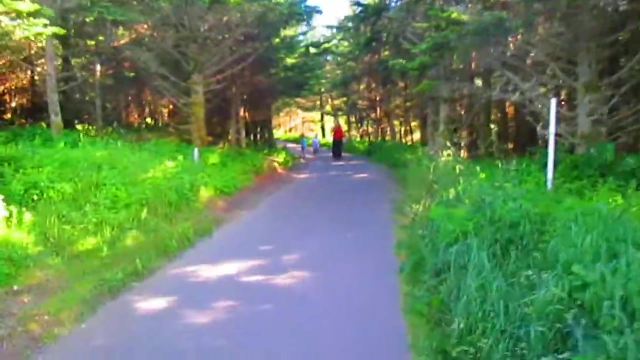 It's a little restaurant. May be have some dinner here. camp here. Might have to camp out in the National Forest someplace. Well, the parking lot ends up here, but you have to walk to the very top. Thanks, Cool. 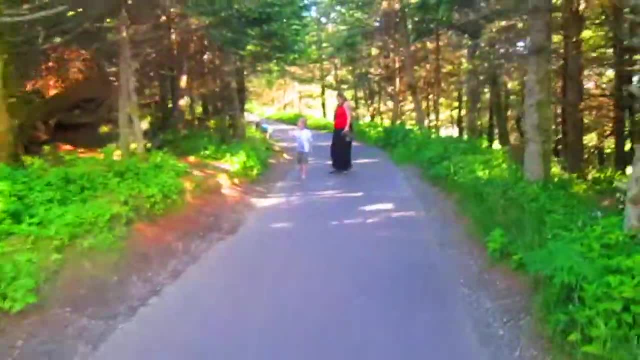 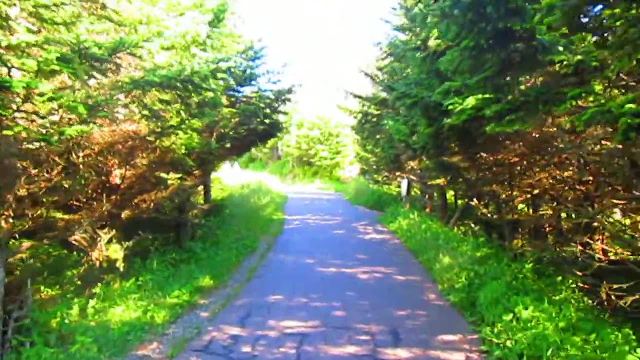 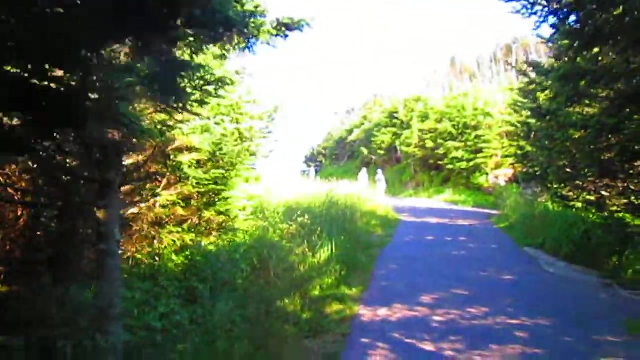 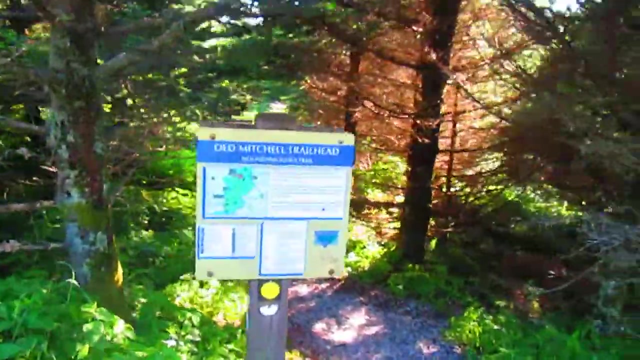 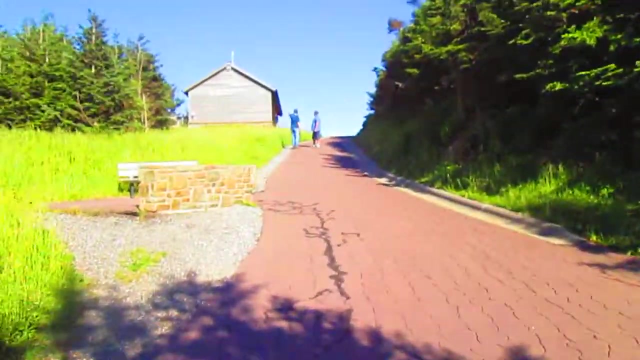 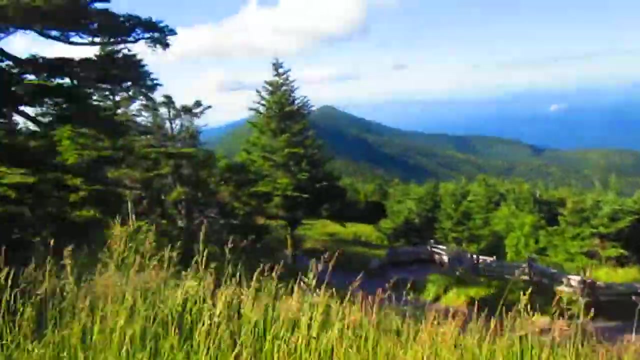 Cool, Cool. Well, it's kind of a fresh walk. This is June, late June, and it is feeling fresh. I put my long sleeve shirt on. Very pretty out here, really Great weather. I'm going to try and get my foot on it.